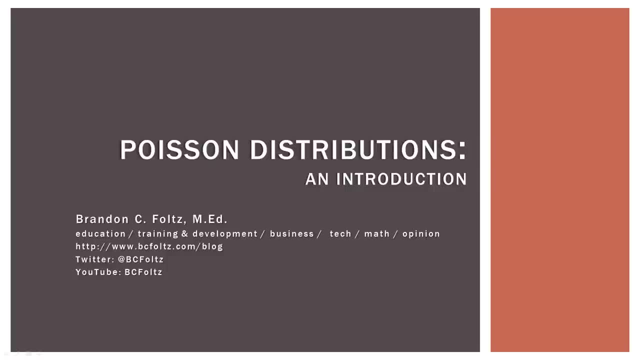 the Poisson distribution. It's not like someone said in the class once, the poison distribution. That did happen. I promise It's the Poisson distribution. So it's very similar to the binomial distribution and actually it's kind of a cousin. 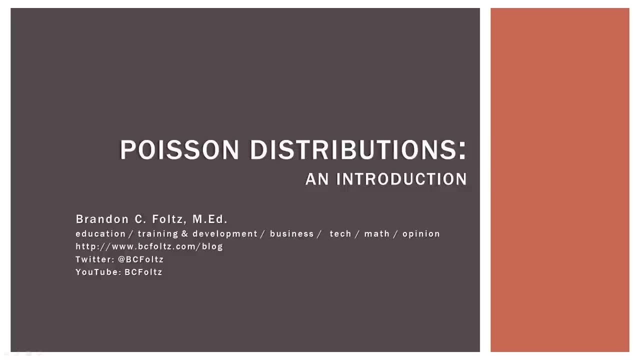 of the binomial distribution. So if you do know something about the binomial distribution, this will make a whole lot of sense, because it works in a very similar manner. Now it's most often used, not only in statistics in certain situations, but also in fields. 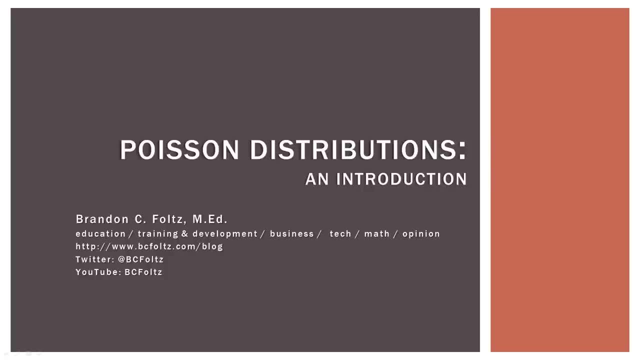 like operations management, Specifically what's called queuing theory And a queue, especially if you're in Britain. a queue is what we call in the United States, waiting in line. So you're in the queue or you're in line. 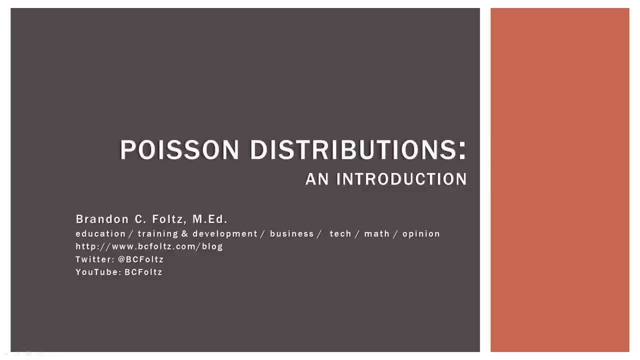 And if you think about that- let's say you go to a bank and you walk into the bank and you get in line- Then, once you're in line, you wait a certain amount of time and then you proceed forward to have whatever 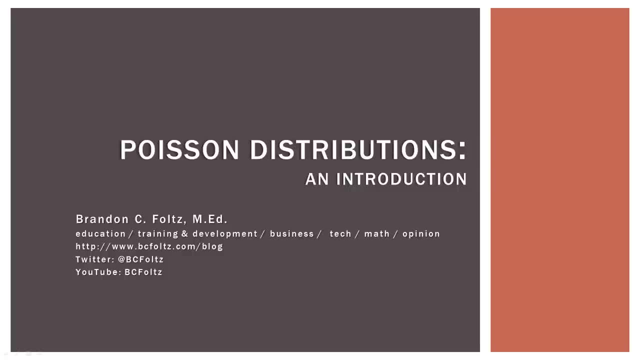 banking services you need, There's a service time and then when you're done with your service, then you walk out. Well, that whole process is called queuing theory in operations management and management science, So this is used not only in stats. 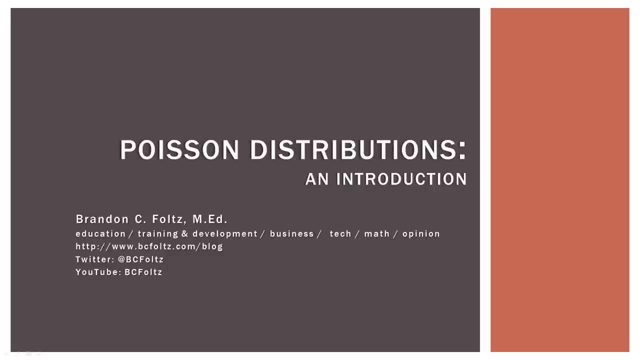 but in other disciplines with very practical implications. And actually the example we're gonna use in this video is a very simplified version of a queuing theory problem or sort of a waiting in line problem. So, all that being said, let's go ahead and dive right in. 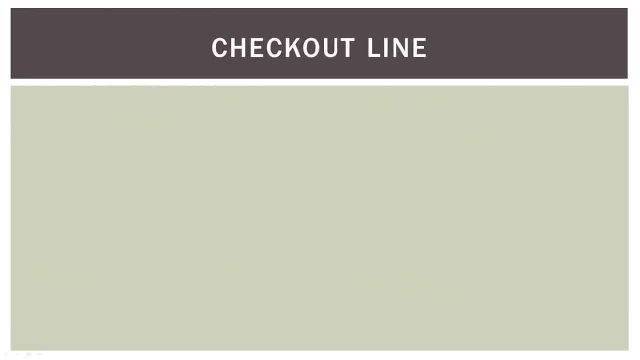 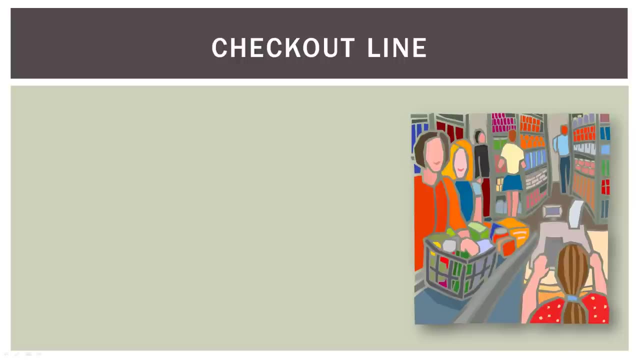 So this is what I call the checkout line example. So there are some people there waiting in the checkout line at the grocery store, and here's our problem. Let's say that you are a cashier at Walmart, It's 4.30 pm and your shift ends at five o'clock. 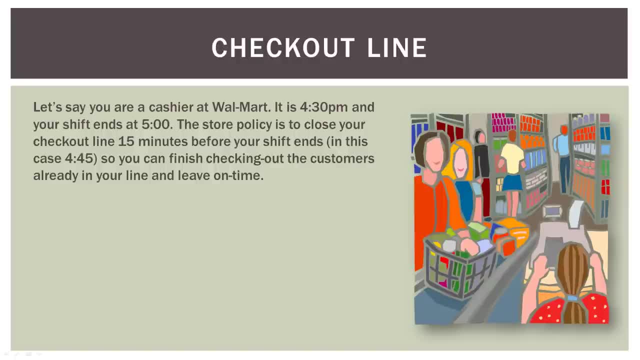 Now the store policy is to close your checkout line 15 minutes before the checkout line ends. So if you're a cashier, you're gonna close your checkout line at 4.45 pm before your shift ends. So in this case, your checkout line should end at 4.45.. 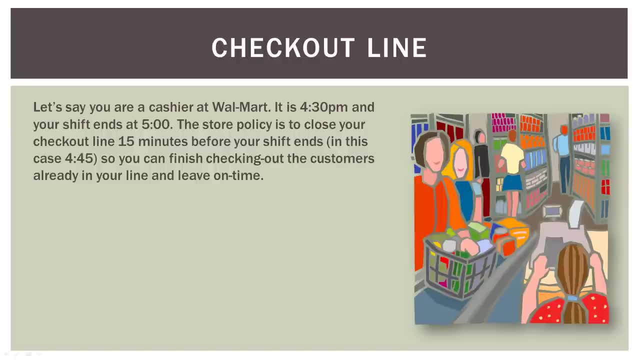 That way you can finish checking out whatever customers remain and of course you'll take your register probably to the office to balance out and things like that. So it's 4.30, you're scheduled to get off your shift at five. 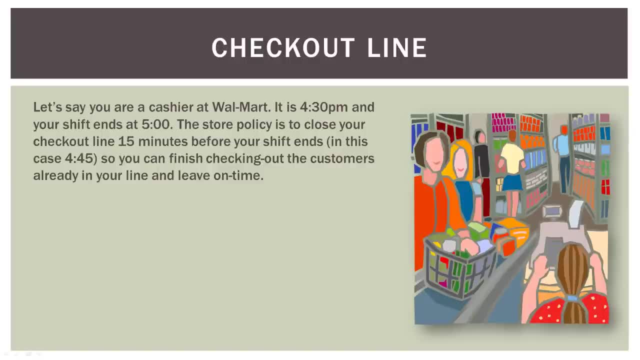 but they're gonna close your checkout line at 4.45 to make sure you get out on time Now, depending on the overhead cameras, like the security cameras in the store, the store data indicates that between 4.30 and 4.45 pm. 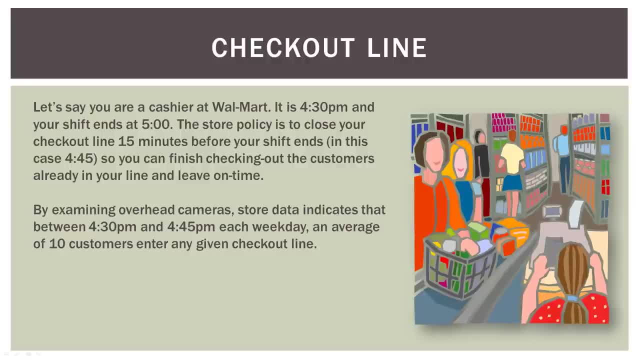 on each weekday- we're gonna assume this is a weekday- an average of 10 customers enter any given checkout line. So you can imagine, as a customer you're walking around the store and you got all the things you need and then you kinda walk up to where the checkout lines are. 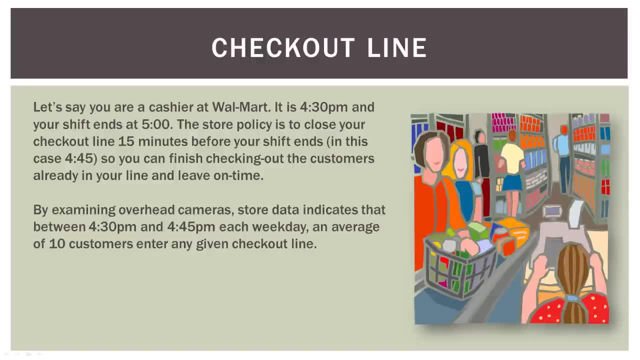 and you decide probably by which is the shortest which line to get in. So once you become part of that line or part of that queue, you know that's what we're considering here. So between 4.30 and 4.45 each weekday. 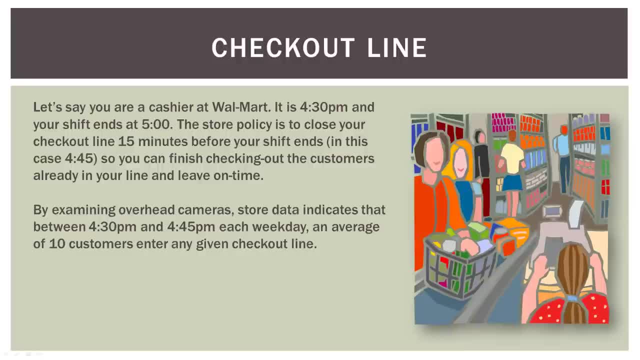 on average, 10 people basically get in line, And that's all we're worried about. We're not worried about how long it takes to check them out or anything like that, just the number of people that get in line. So here are two questions we're gonna use in this video. 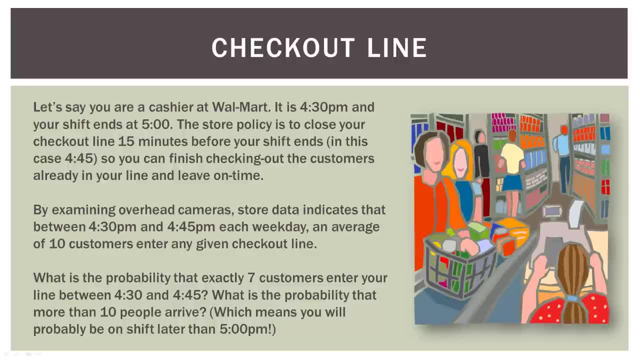 What is the probability that exactly seven customers enter your line between 4.30 and 4.45?? Another question we're gonna answer: what is the probability that more than 10 people arrive into your line between 4.30 and 4.45?? 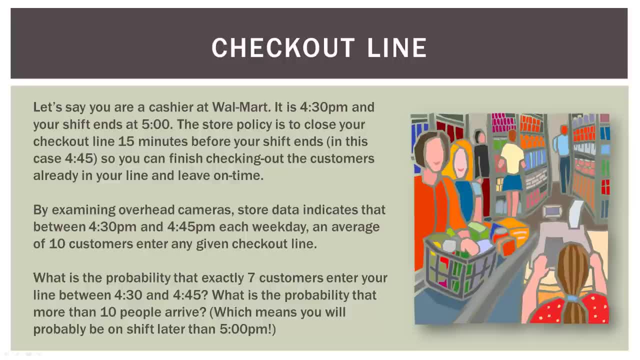 Now remember, on average, or we're expecting 10 customers to come into our line during that 15 minute period, But we're gonna look at the probability for exactly seven and then the probability for more than 10, which is more than we would expect. 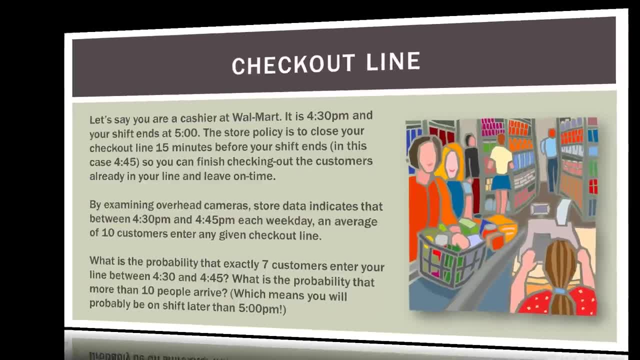 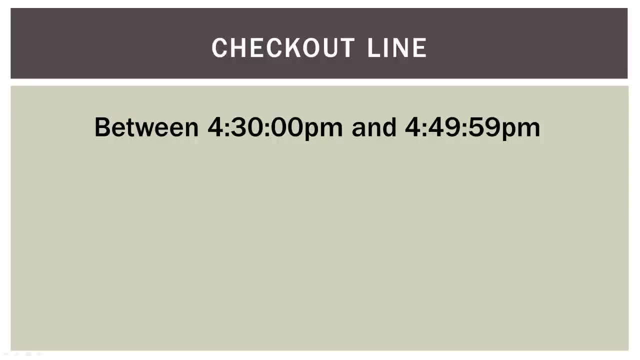 Of course that means you probably would not gotta work on time. So here's our time frame between 4.30 pm and we're gonna say 4.49 and 5.59.. I'm not gonna include the exact 4.45,. 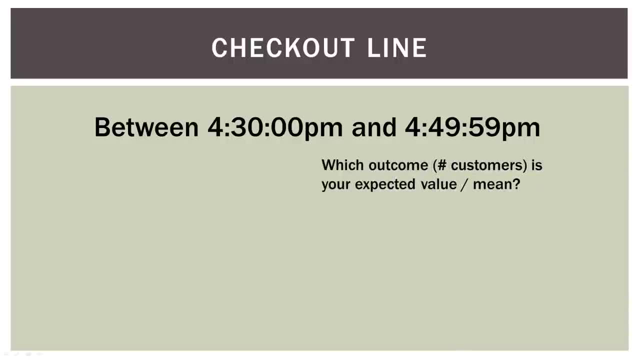 but it's really not important. Now here's the question I want you to answer with your intuition: Which outcome, so the number of customers that get in line, is your expected value, or sort of the mean number that come, And actually you should already know this. 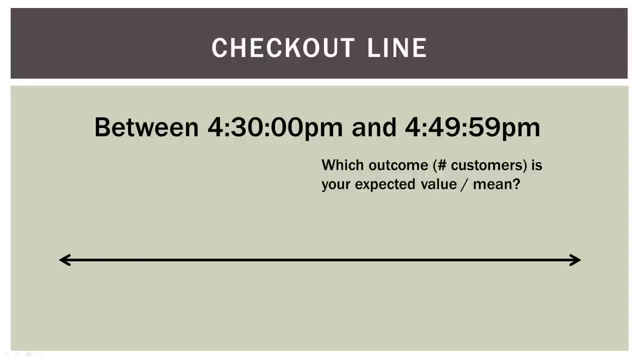 it was in the question. So we have a continuum here and we could have zero customers during that 15 minute period. That's probably not that likely, but it could happen Theoretically. theoretically we could have an infinite number of customers come into our line. 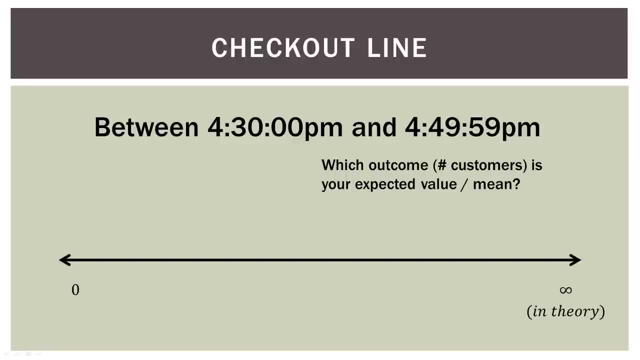 Now, is that actually gonna happen? No, But that's why it says: in theory, That's part of the Poisson distribution. it could theoretically go all the way to an infinite number. Now that actually gonna happen? That's part of the Poisson distribution. that could theoretically go all the way to an infinite number, to several customers in line. Let's say we get a 12 number that are coming in. Let's say we get a 14 number that's only from this line And another 15 number would also come to our line. 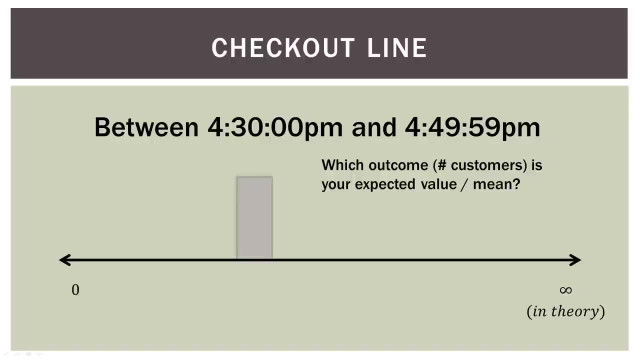 number of customers, but of course that's not going to happen. Now, what number of customers would you expect? Well, it's not a trick question, Because, remember, in our problem it said we would expect 10 people to get in line. 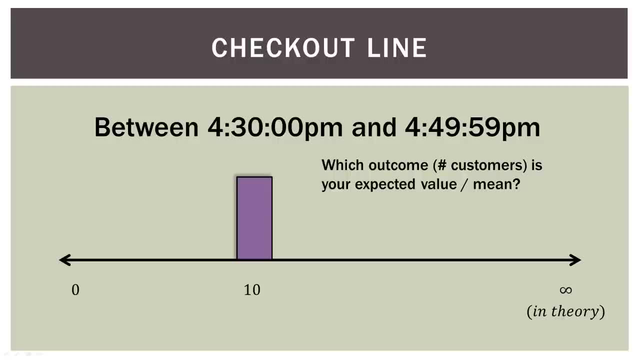 That's what the store figured, the average was. So that is our expected value, That is our mean value And in these type of problems, the expected value- remember the expected value- is just the mean of a discrete probability distribution. So expected value and mu, the symbol mu there. 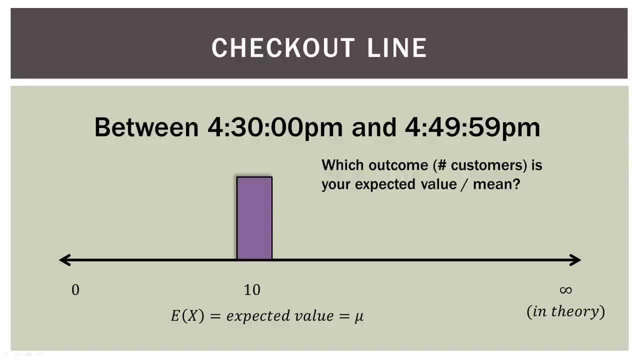 the mean are really the same thing in these type of problems, So don't get confused. they mean the same thing. But again, we would expect 10 customers in that 15 minute period. Now, if you graph that in Excel, 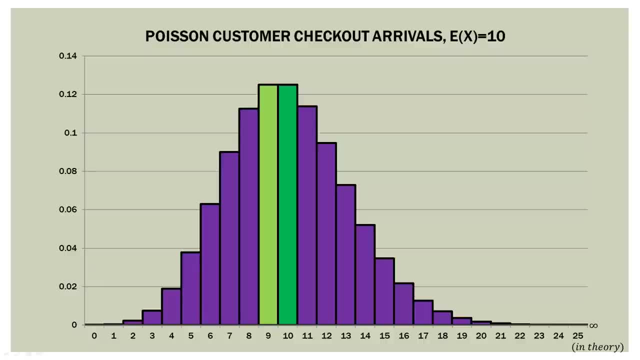 and I'm gonna do that in a different video to show you how I got this graph. you will see that on the left-hand side we have zero customers coming into our line. That's the x-axis along the bottom. That's the number of customers. 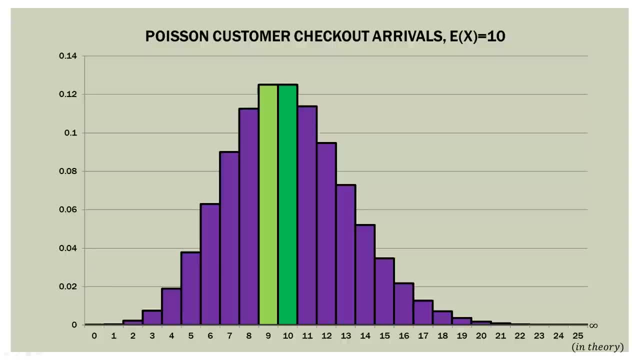 Along the y-axis. the vertical axis is the probability associated with each outcome. So you can see that down at the left-hand side, we have the probability of zero customers. Well, that's not that likely. As you can see, the bar is very, very, very, very short. 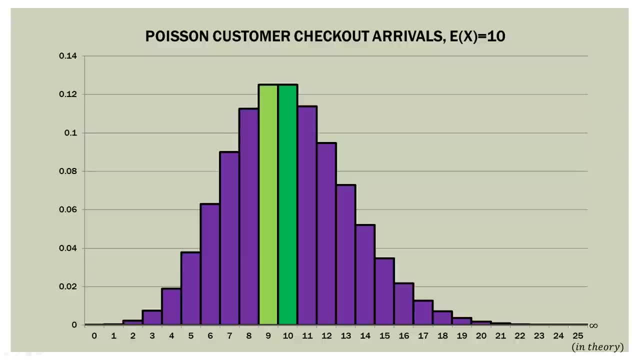 It's very small. There is probability there, but it's not very much. And of course, as we go up the number of customers, the probability gets higher and higher and higher. So if you look at 10, which is the dark green bar there, 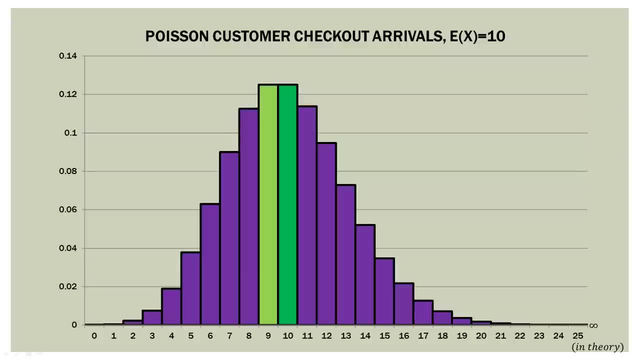 remember that was our mean. We can see that the probability there seems to be about .125, you know somewhere in there. But also the probability for nine customers is the exact same, And sometimes that happens in these discrete probability distributions. 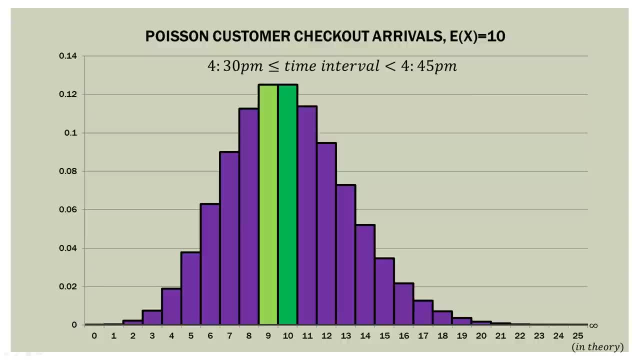 So remember, this is for our time interval of 4.30 to 4.45.. Now, even though nine customers and 10 customers have equal probabilities, the mean or expected value is still 10.. It just means that the probability. 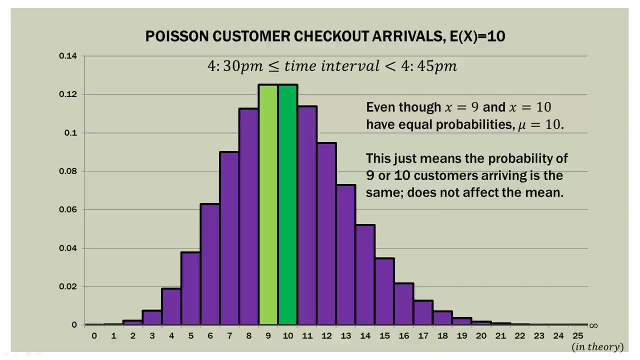 of nine or 10 customers arriving is the same. It doesn't affect the mean in any way, And that's just what sometimes happen in discrete probability distributions. But just remember, the height of each bar is the probability for that outcome. Now, as you can tell, as we go past 10,, 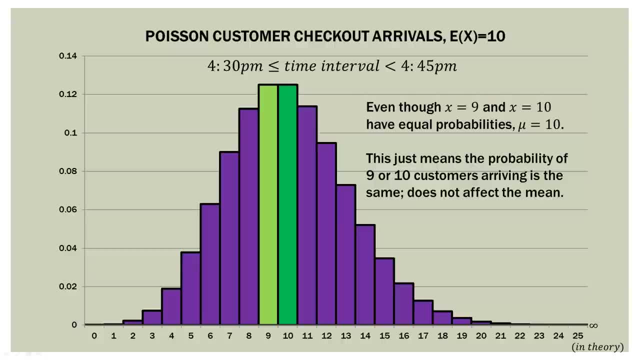 and then on to 11,, 12,, 13,, 14, number of customers. the probability keeps going down again Again. in theory this goes all the way out to infinity. It's kind of a limit problem. So if you've done other mathematics, 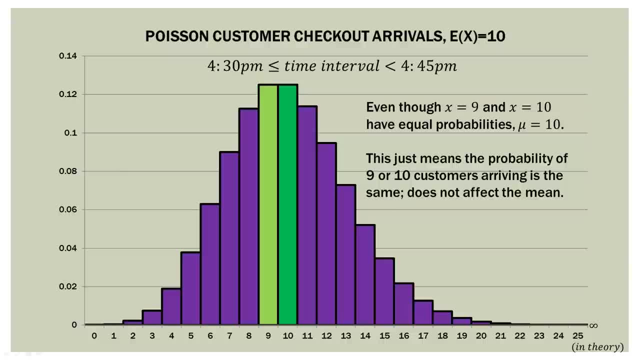 you kind of understand what limits are, But it never really, you know, gets anywhere. It theoretically goes to infinity And the probabilities become so small that they are basically zero. Okay, so you can see that this distribution is very similar looking to binomial distributions. 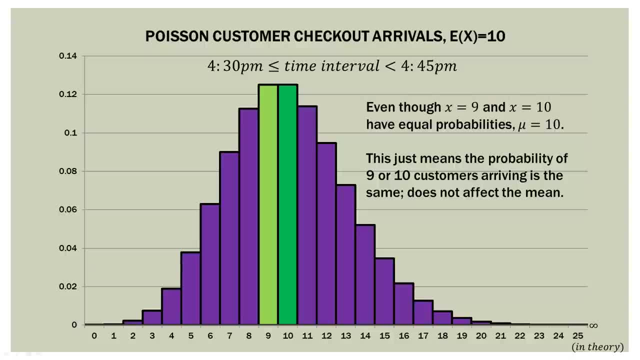 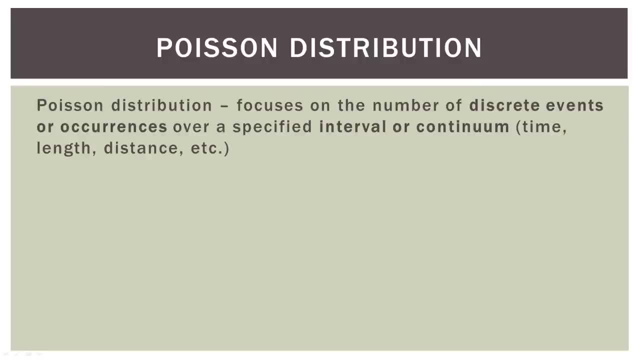 And that's not really by accident, because they are related. They're not the same, but they are related. So let's talk about a formal definition here: The Poisson distribution. What it does is it focuses on the number of discrete events or occurrences. 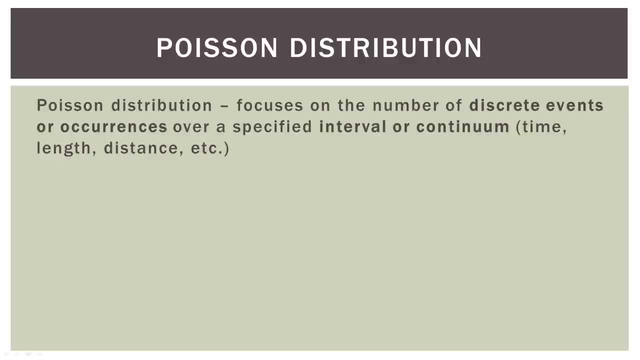 over a specified interval or continuum- That could be time, length, distance or whatever It's over some continuum And the number of events that happen only within that interval. And that's what makes the Poisson what it is: Number of events in a specified interval. 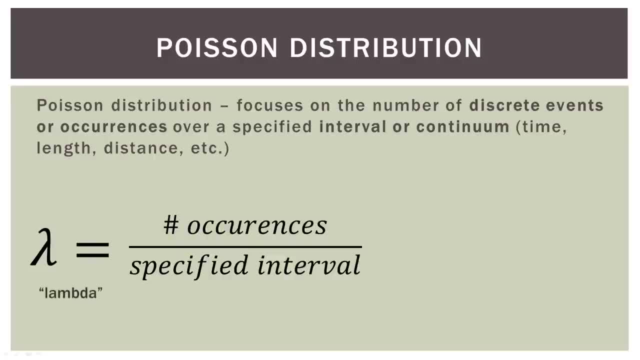 And we have a new symbol for that. It's called lambda. So in the Poisson we have a new symbol that at least we haven't used in my videos. So it kind of looks like a- I don't know a little triangle thing. 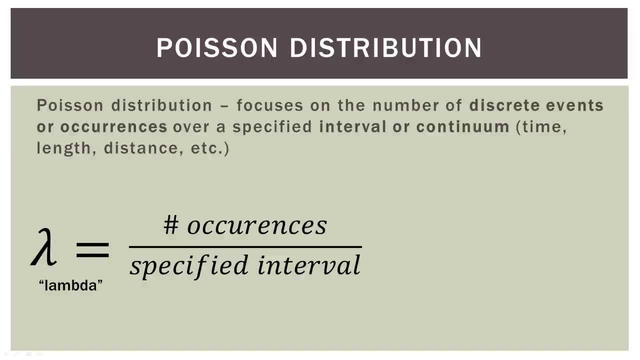 But it's the Greek letter lambda, And that is just the number of occurrences over the specified time interval. And again, this is what you know. you can get symbols mixed up, but lambda is the same thing as the expected value or the mean. 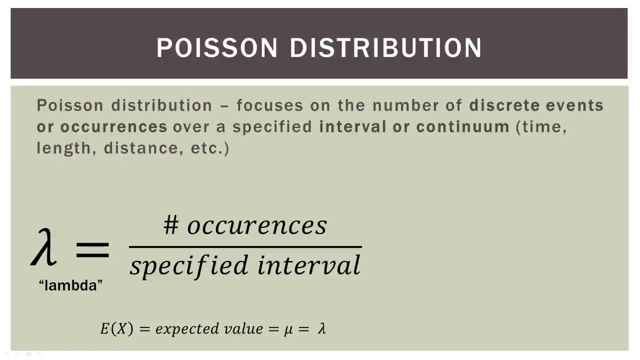 These all kind of mean the same thing. You could actually substitute them in, and actually I'll show you that in a minute, and it doesn't change the meaning: They are the same thing. So let's look at our checkout line example. 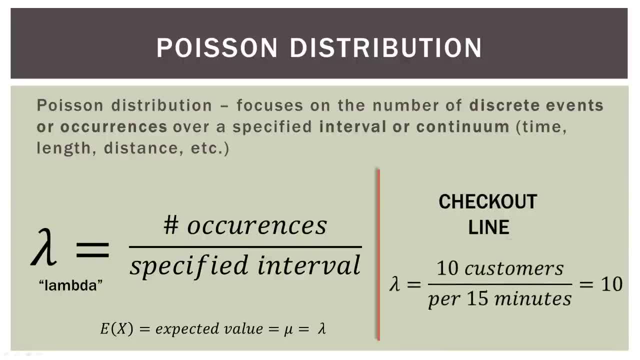 Lambda in that case is that we have 10 customers per 15 minutes, So our lambda here is 10.. Now it's important to point out there that's not a fraction. you're going to simplify. I mean you could, but it would change. 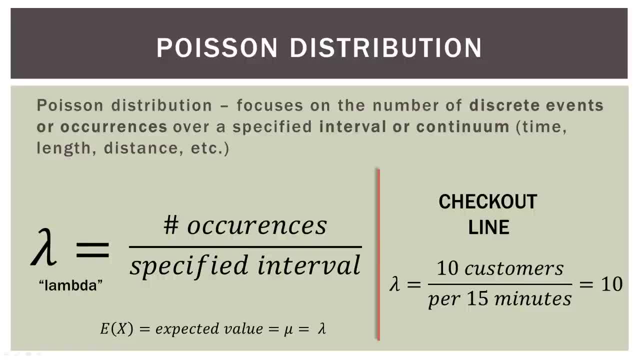 It would be like two customers every, you know, three minutes or something like that, But we're talking about a 15-minute interval. That is the interval we decided to have. That's the interval we decided to have. That's the interval we decided on. 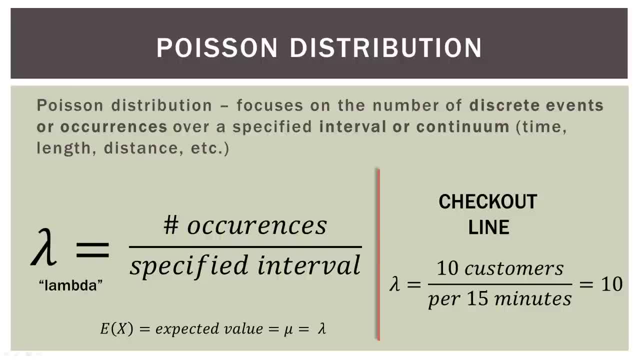 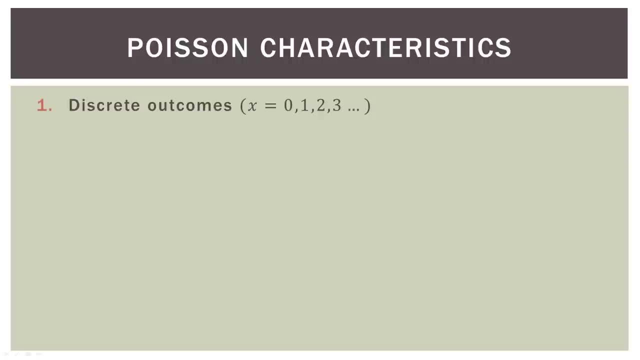 And 10 customers are expected during that 15 minutes. So our lambda here is 10.. So do not try to simplify that, because we're interested in our 15-minute period. So let's talk about a few characteristics more formally. Just keep in mind that the Poisson is discrete outcomes. 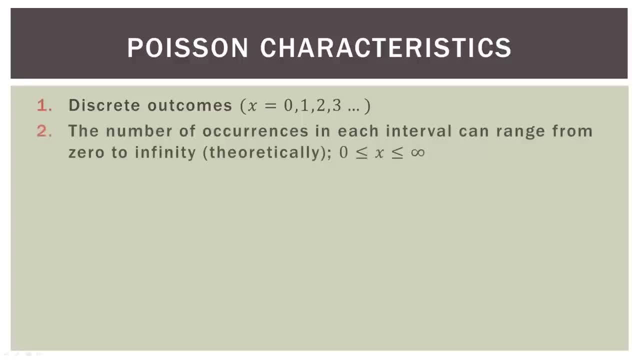 So zero, one, two, three, four, et cetera. The number of occurrences in each interval can range from zero all the way to, theoretically, infinity. It describes the distribution of infrequent, rare events. Each event is independent of the other events. 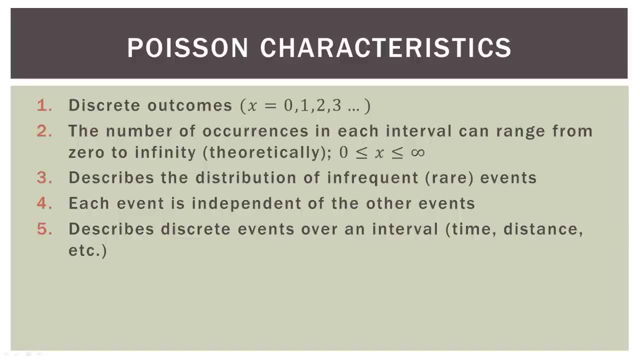 Describes discrete events over an interval, which we already talked about. That's kind of what makes it what it is. That's kind of what makes it what it is. That's kind of what makes it what it is. And the expected number of occurrences. 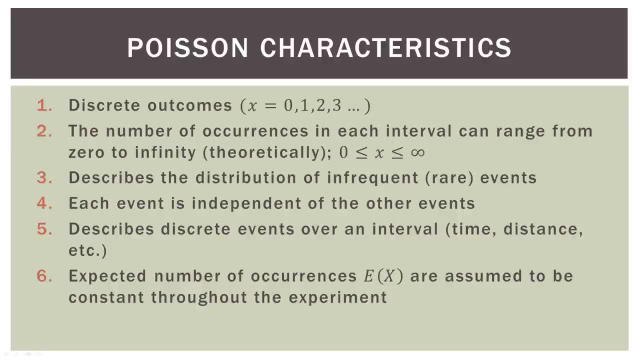 are assumed to be constant throughout the experiment. So this is something we kind of assume. So think about our example: During a 15-minute period we expect 10 customers, So we kind of assume that those 10 customers arrive to our line evenly. 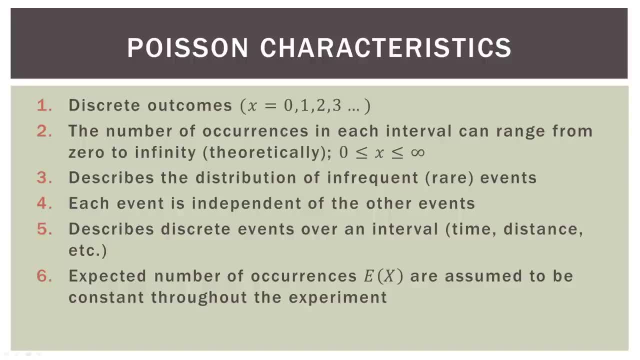 Now, is that actually gonna be the case in real life? Probably not. Now there are types of queuing problems that you can have a constant arrival rate- and I can- or a constant service rate. And as far as a constant service rate, 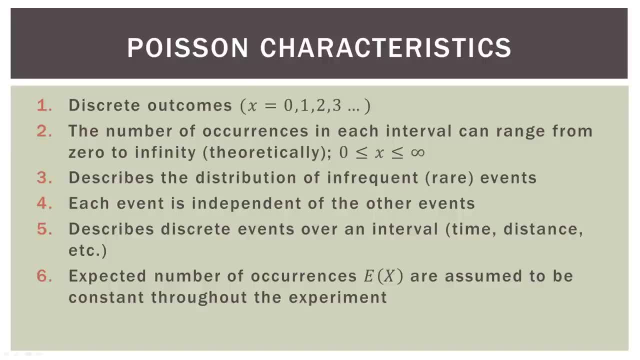 I'll give you an example right now, And that is the automatic car wash. So when you drive your car into a car wash- at least here in the United States- your car moves along that car wash at a constant speed And every car goes through it at the same speed. 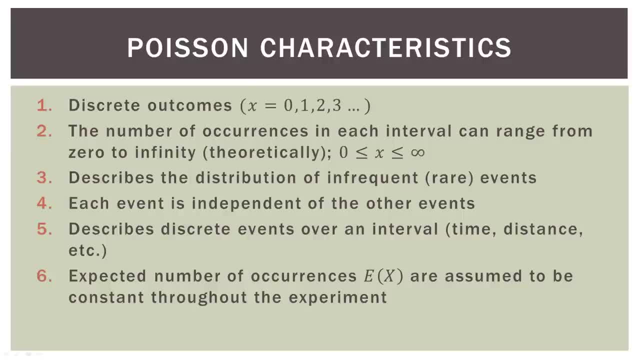 So in that case the service of the car wash is constant, no matter what car goes through. But in our checkout line people are gonna arrive sort of at different times, But for this interval, as long as we're dealing with this interval, it really doesn't matter. 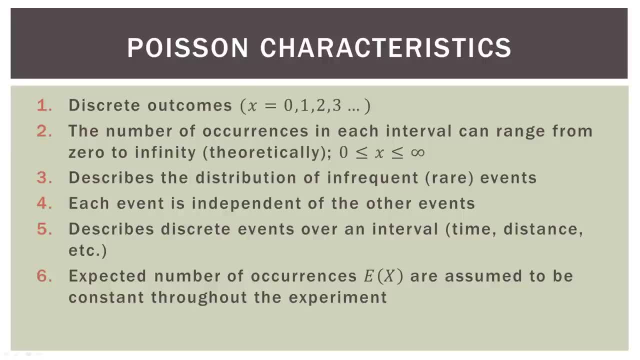 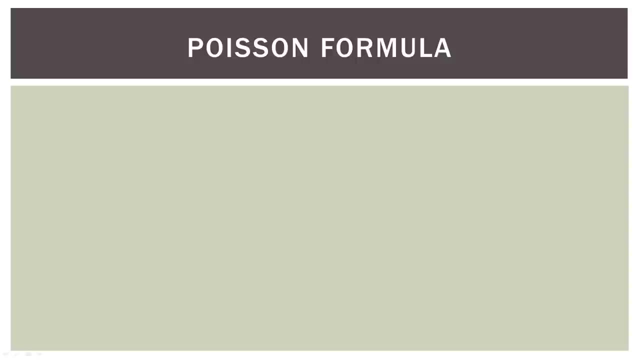 We're kind of assuming that everyone arrives at even times, So just keep that in mind. It's not really that important, but it is just a characteristic of the Poisson distribution, So of course there's a formula that goes along with it. 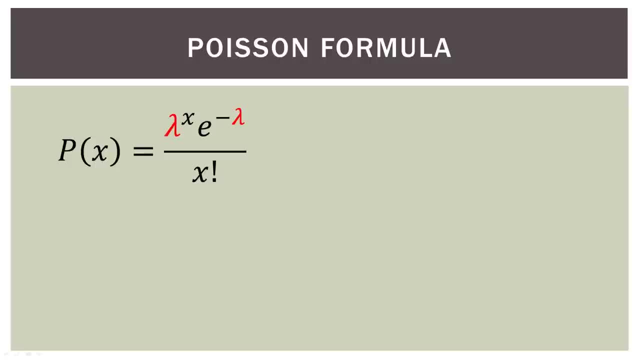 And here's what it looks like. Now, that's kind of crazy looking, but I don't want you to freak out, It's actually fairly simple. So here we have the probability of an outcome x. So we could say: seven customers, 12 customers. 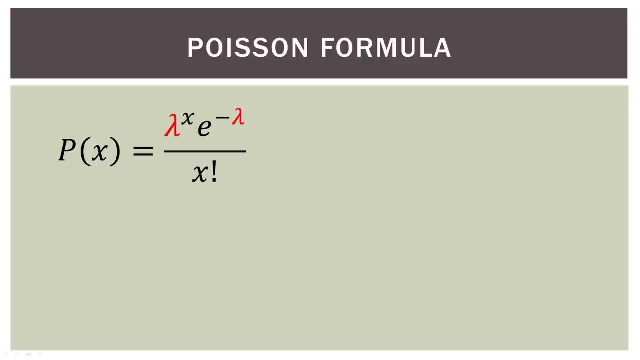 and that would be what x would be. That equals lambda raised to that x power multiplied by e, which is a constant- okay, we'll talk about that in a minute- raised to the negative lambda power divided by the factorial of x. Or it can also look like this: 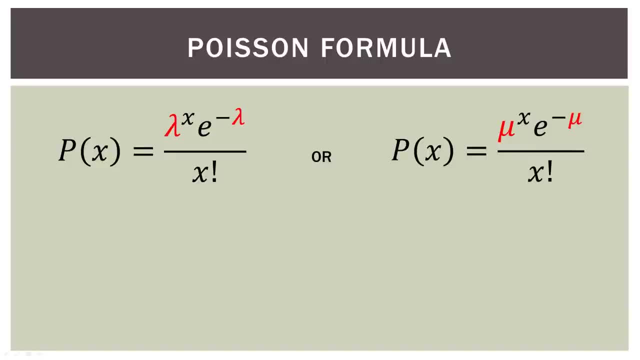 In some books you'll see it this way, where instead of lambda they use mu. But remember what I told you a couple of slides ago. They're the same thing. Now, more formally, lambda is the formally correct way, but I have seen it with mu in place of lambda. 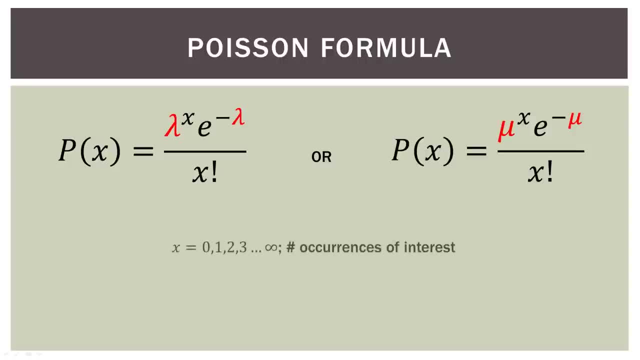 but it doesn't change the meaning. It's the same thing. So x could be one, zero, one, two, three, four, all the way up to infinity. That's the number of occurrences we are interested in. So in our problem, the first question: 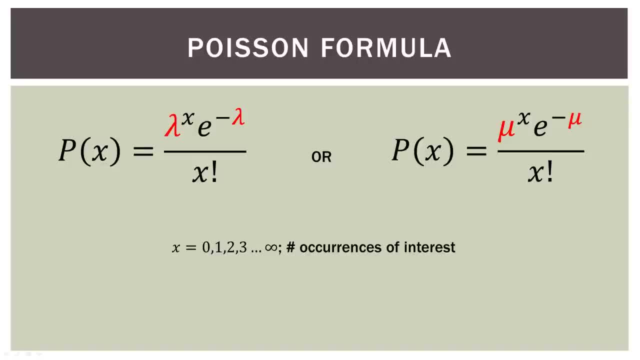 we're interested in seven, So x would be seven. in this formula, Lambda or mu, is the long run average, which is the same. It's the same thing as saying as the number of occurrences we have in whatever interval we specify. And then e is the constant. 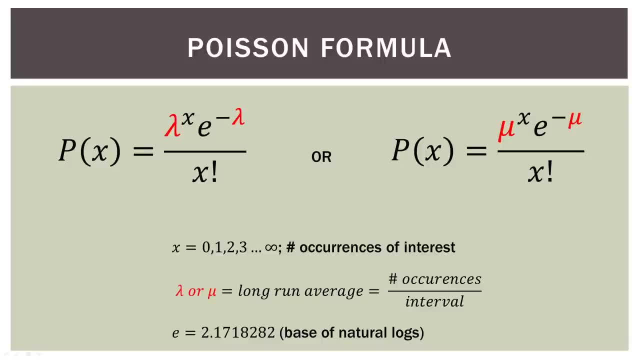 Remember, if you have this- haven't had this since high school or whenever- it's that 2.1718 number which is the base of natural logarithms. So it's that button on your calculator that says e Okay, it's just a constant. 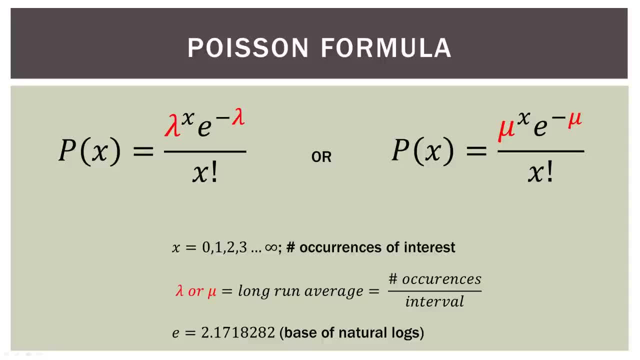 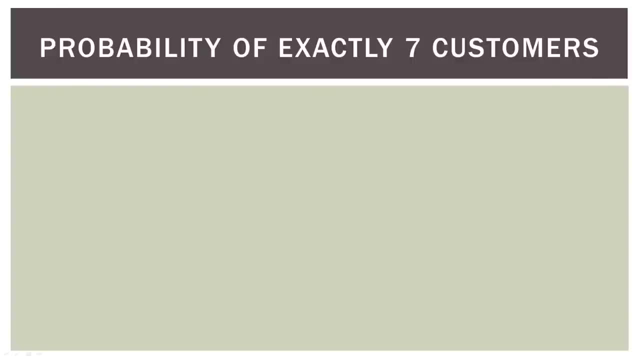 So all we have to do is plug in or substitute. We substitute our numbers into this formula to find our probability. So let's solve our first one: What's the probability of exactly seven customers? So here is our formula. I'm gonna use the lambda version. 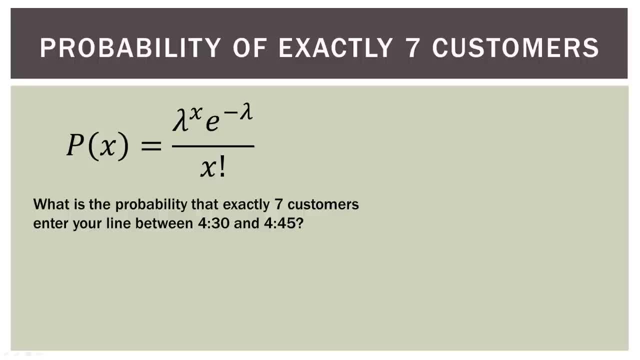 So what is the probability of exactly seven customers that enter your line between 430 and 445?? So x, here is seven, Lambda is 10, because, remember, we're expecting 10.. That's our average. That's our average, our long run average. 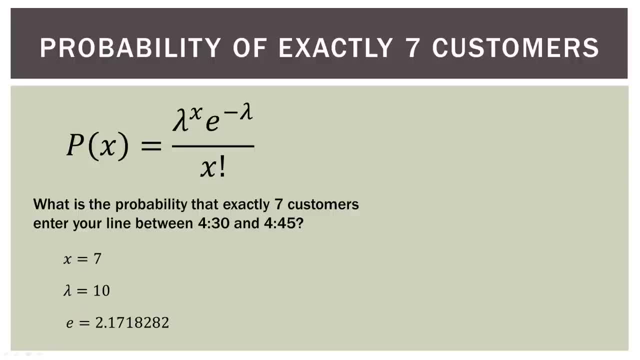 And then e is a constant. It's always e, So 2.1718.. Now we substitute those numbers into our formula here. So lambda is 10, and x is seven. So 10 to the seventh multiplied by e to the negative 10,. 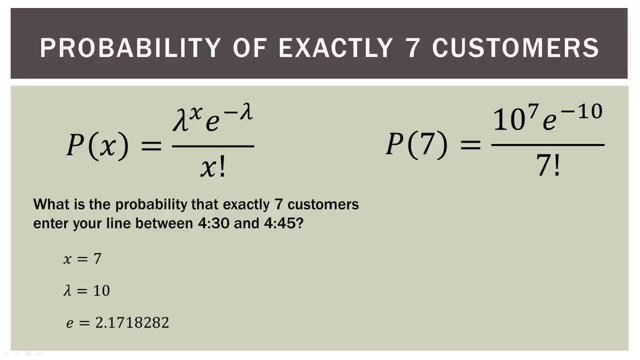 because it's e to the negative lambda divided by seven factorial, And that's because seven is our x. Now, when we do that in our calculators, we come up with 0.09, which of course is 9%. So the probability that exactly seven customers. 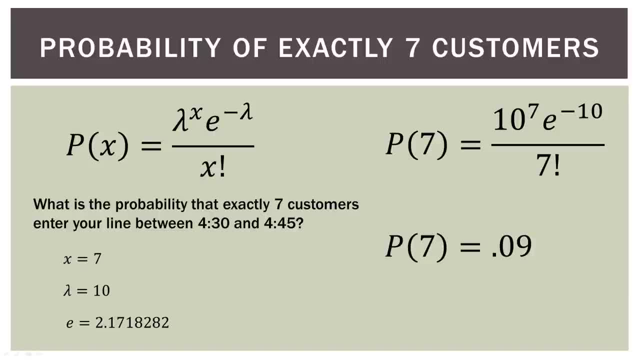 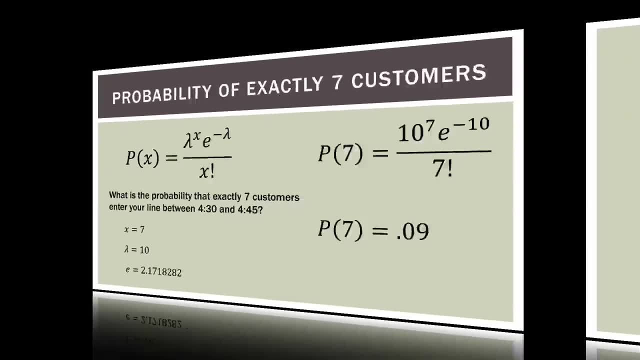 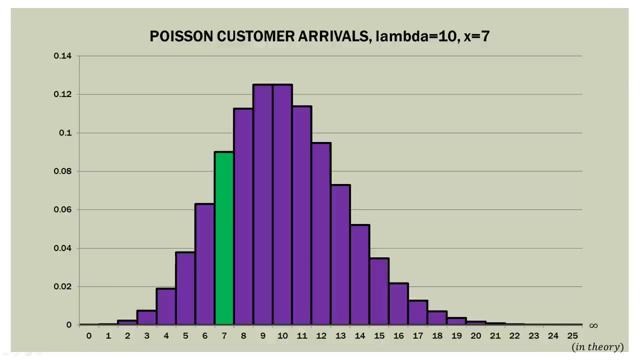 come to our line between 430 and 445 is 9% or 0.09.. Now, if we go back to our graph, here we have at the top there we have lambda equals 10, and x equals seven. That's what we're interested in. 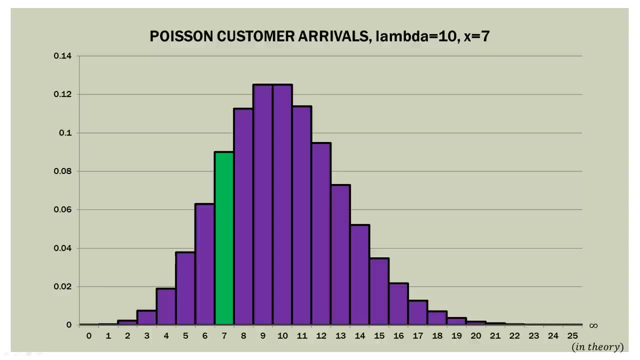 So if we go over to the seven bar in our graph, I've covered that in green so you can see it. If we go over to our axis, look where it meets up at 0.09.. So we can use our graph to check our calculation. 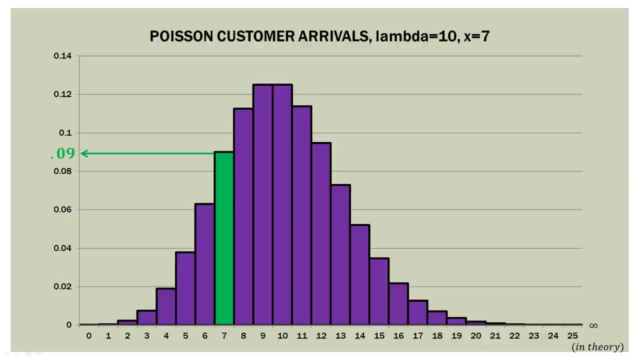 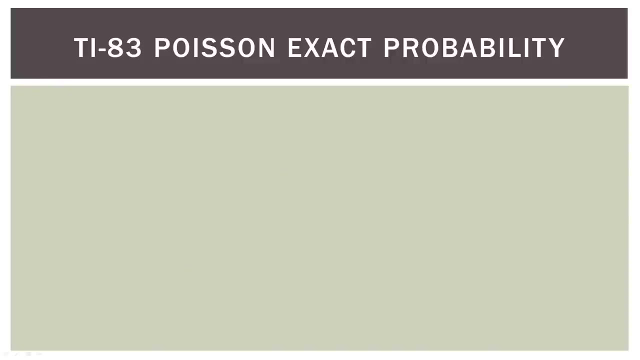 And they both concur, so we know it's correct. The probability of seven customers coming into our line in that 15 minute interval is 0.09.. Or nine percent. Now, there is a way to figure this out in a TI-83 calculator. that's what I use. 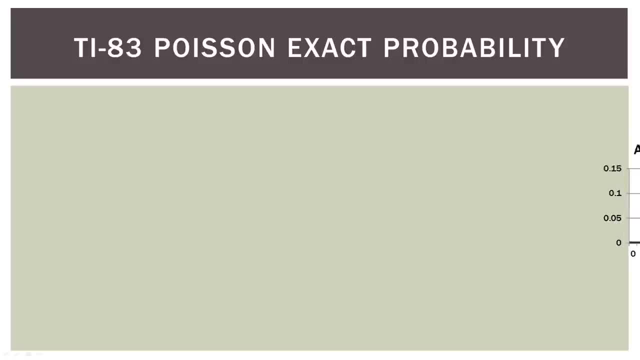 I have a TI-83 plus, but I'm sure this is the same for all the TI models. So here is our graph and again we're interested in the height, or the probability, which is the same thing, of that green bar. 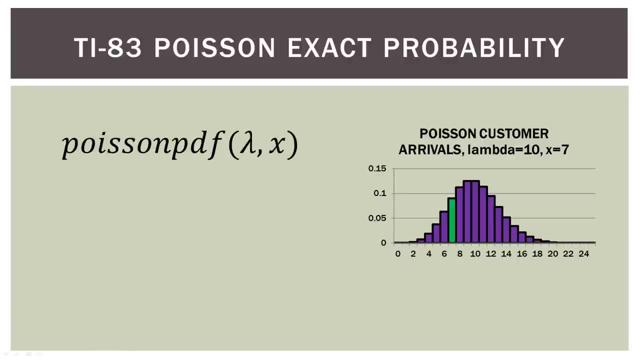 which is x, equals seven. Now the function in the calculator is the Poisson P, D, F function and it requires two arguments: Our lambda and the number of occurrences we are interested in. So to find that you just press the second. 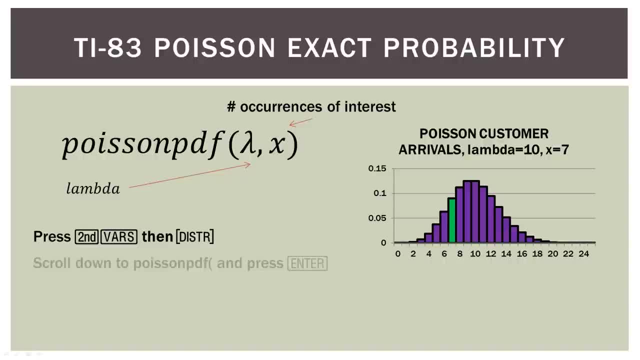 in the vars button. that takes you to the distribution menu. You'll scroll down and you will find the Poisson P, D, F function. press enter. Then you type 10 comma seven, which will put the command in your calculator, so it'll say Poisson. 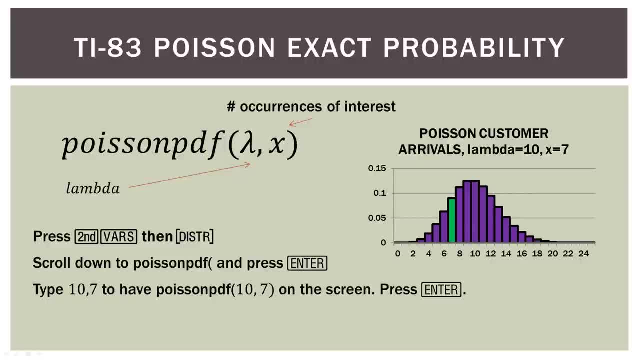 P, D, F, 10 comma, seven, and then of course press enter. That will give us the exact probability of x equals seven and it comes back 0.09.. So you can find this exact probability in the TI-83 or TI-84,, I'm sure, 85 and 89 calculators. 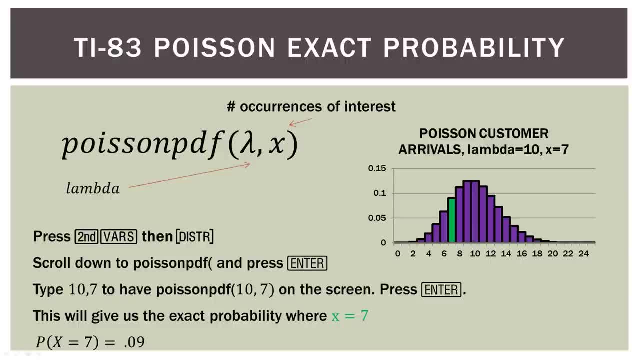 Now a couple of things to keep in mind. if you do this on your calculator Number one, it's very easy to accidentally select the binomial P D F function, because they're basically right next to each other. So always make sure you're selecting the Poisson P D F. 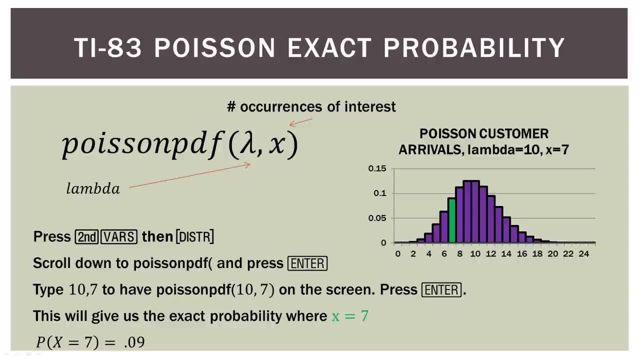 when you're finding an exact probability. Now, on that note, this command in the calculator is for finding the probability of an exact outcome, So exactly seven, Or exactly 12, or exactly four, or whatever else. We're gonna talk about the Poisson C, D, F function. 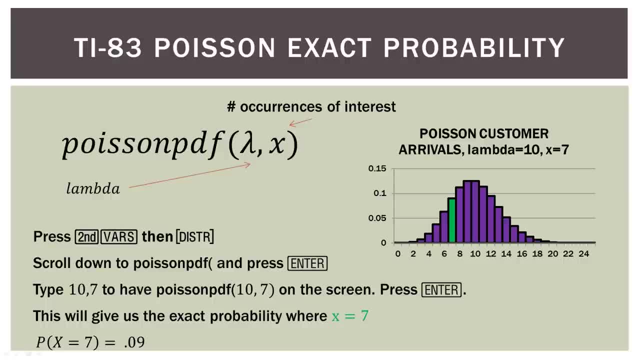 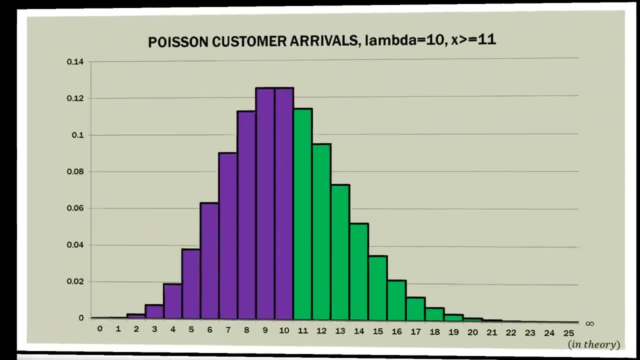 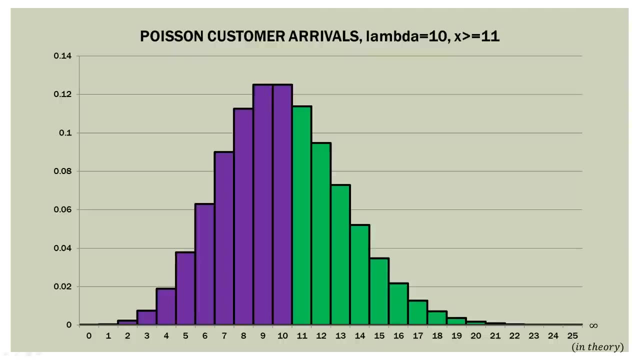 here in a minute. So P D F is the specific probability of any specific outcome. Okay, now remember the second part of our question. What is the probability of more than 10 customers arriving? Well, if you look at this, 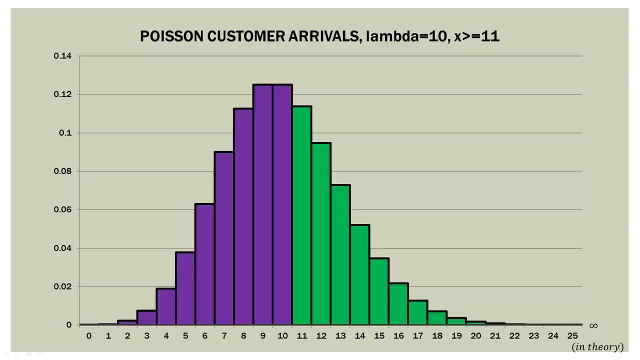 anything more than 10 would include 11,, 12,, 13,, 14,, 15, so on. So we're interested in the green part of our graph here. But how do we find that? Well, if you remember, in the binomial videos. 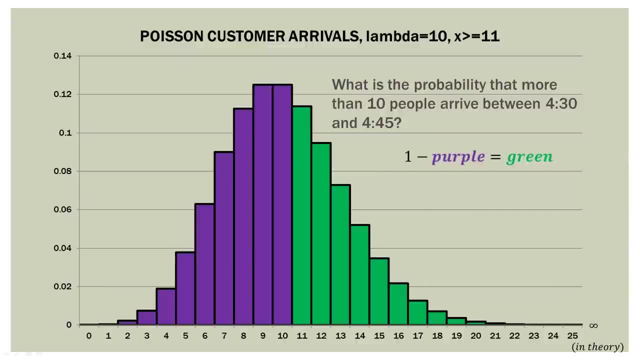 I did something very similar, So remember that the entire probability distribution has to add up to one. That's just sort of the law of probability distributions like this. So if we wanna find the green, what we can do is we can take one. 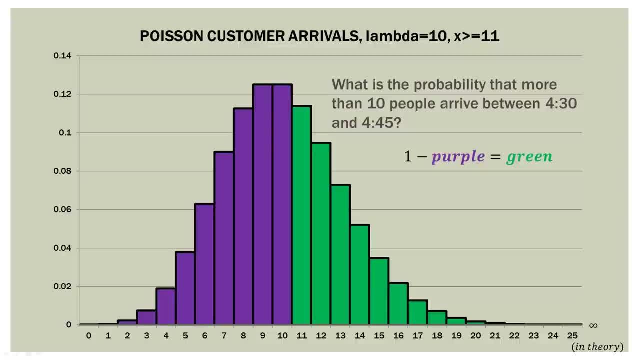 which is the whole, and then subtract or sort of chop off the purple, and that will leave us with the green. So we can sort of do a puzzle here and figure out the green by subtracting the purple part from one. So how do we do that? 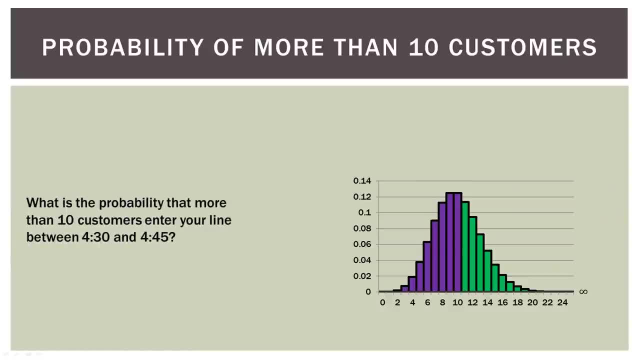 So here's our graph. So what's the probability that more than 10 customers enter your line between 430 and 445?? So here's our formula again. Now, x is 10.. Now, why is that? Why is our outcome of interest 10?? 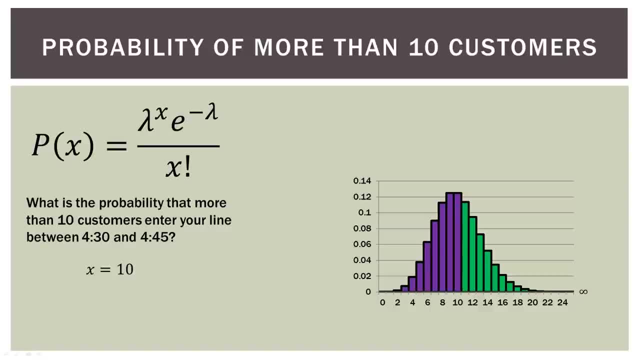 Well, if you look on our graph, that is the upper limit of the purple region. we're gonna wanna subtract out. So we're gonna find the purple area and subtract it from one. So x, in this case is 10.. Lambda is always 10 for this distribution. 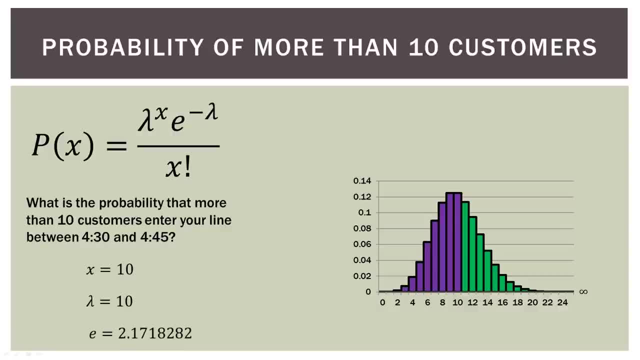 And then when I say that lambda is always 10 for distributions of this problem, So it can obviously be different for different problems. So e is the constant 2.1718.. So now we can go ahead and do this So to find the green part. 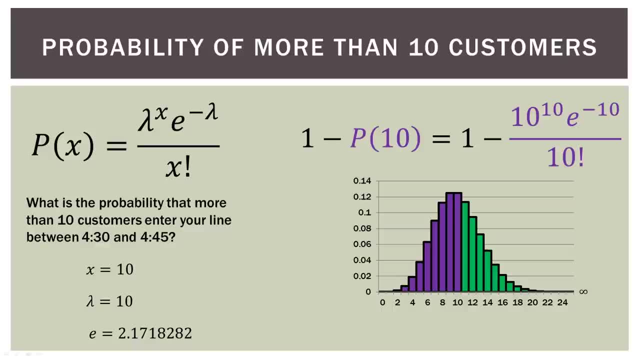 we take one minus the probability, all the way up from zero. minus the probability all the way up from zero. minus the probability all the way up from zero, zero to 10, and I'll show you how to do that here in a second. 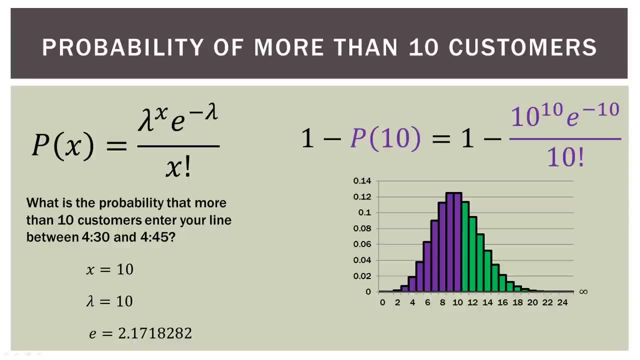 So we go ahead and subtract that purple part out and we have one minus .583 equals .417.. And that is the probability of the green part of our graph. Now I do want to point something out here, which I'll show you in the next slide. 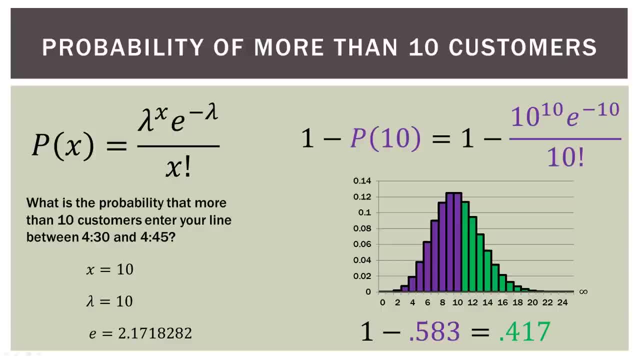 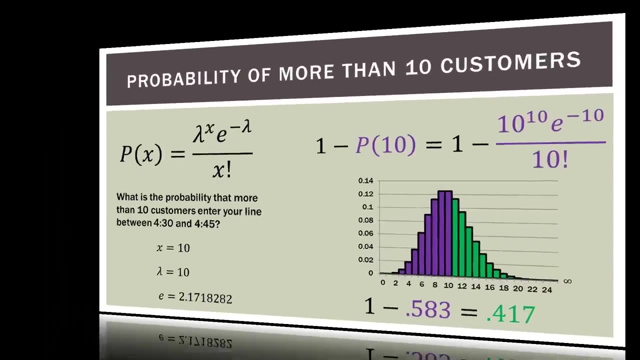 Remember to find the cumulative probability there in the purple In our calculator. we will not use the Poisson pdf function, We're gonna use the Poisson cdf. But I'll show you that in the next slide. So here's what we're trying to find. 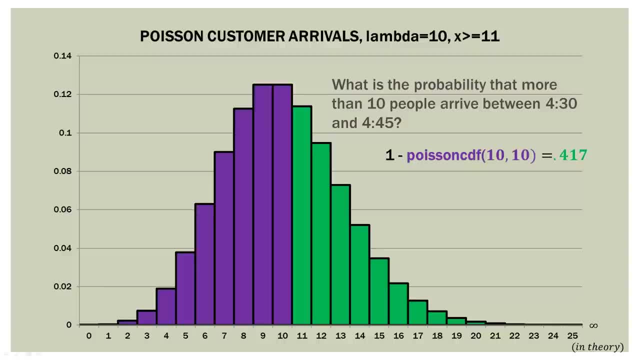 And the function we want in this case is the Poisson cdf, And the c in that case stands for cumulative. So the cumulative will give us the probability all the way from zero, all the way up to 10.. So one minus that will give us the green part. 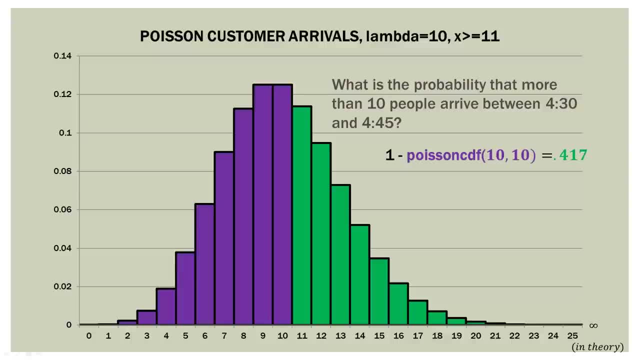 So just remember, the pdf version of the function gives us an exact probability at any given exact outcome. The cdf gives us the cumulative all the way from zero up to whatever number we specify, In this case 10.. So we go ahead and do that subtraction out. 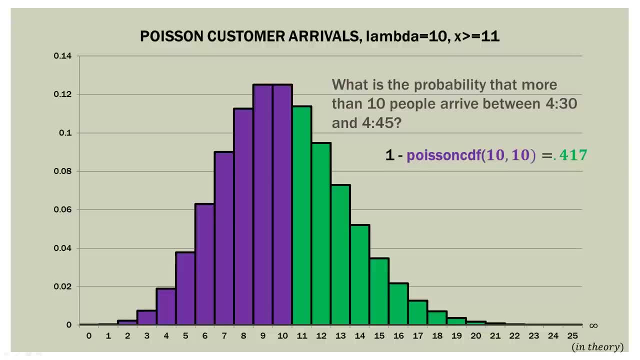 And the whole area of the green is .417.. Which means the probability of more than 10 people arriving into our checkout line between 430 and 445 is 41.7%. The probability of more than 10 people arriving into our checkout line between 430 and 445 is 41.7%. 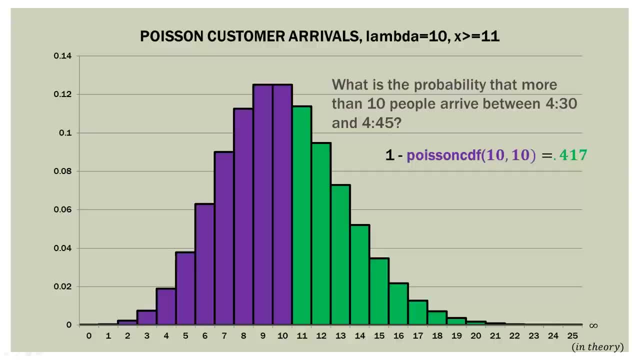 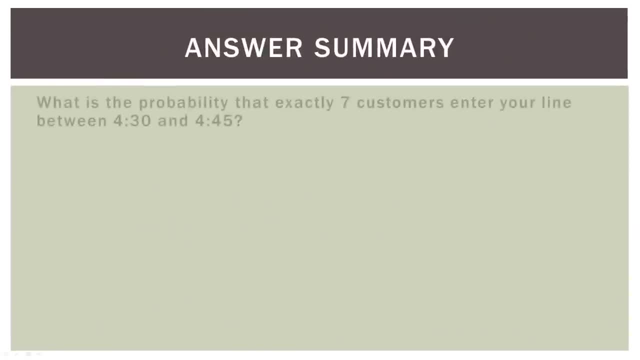 That's a pretty good probability, or a pretty good percentage, as far as more than 10 people coming into our line during that time. So our answer summary: What is the probability that exactly seven customers enter your line between 430 and 445?? 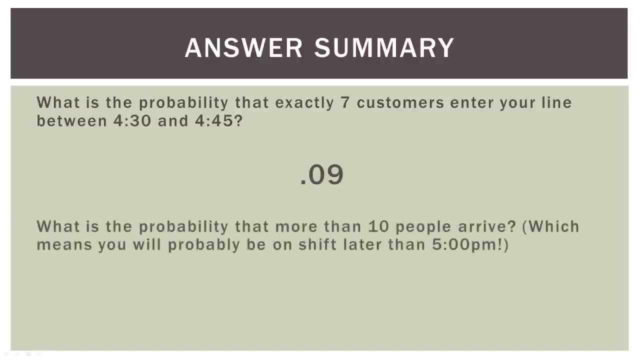 Well, it's .09,, which is nine percent. What is the probability that more than ten people arrive? Well, that was .417 or 41.7%, 7%. So again, these are just the probabilities of these specific outcomes, given the time interval we're interested in. 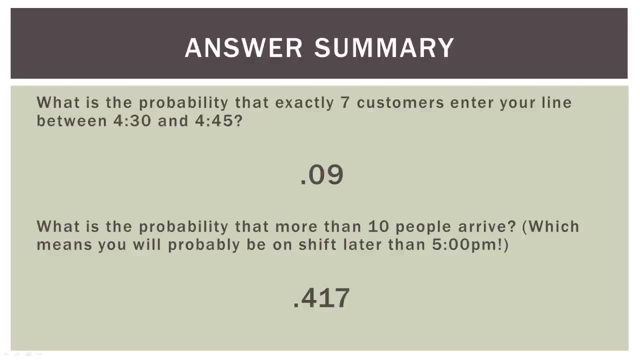 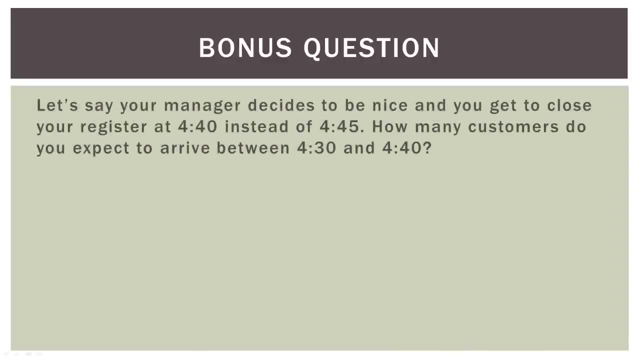 and the number of people we expect, the mean number of people we expect to come into our line, based on some previous data we have or calculated. So finally, a bonus question. Let's say your manager decides to be nice and you get to close your register at 4.40. 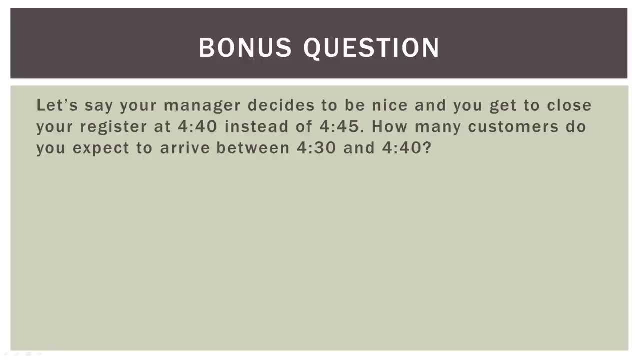 instead of 4.45.. How many customers do you expect to arrive between 4.30 and 4.40?? So here is our change. we gotta do. We expected 10 customers in that 15-minute interval. What if we change it to a 10-minute interval? 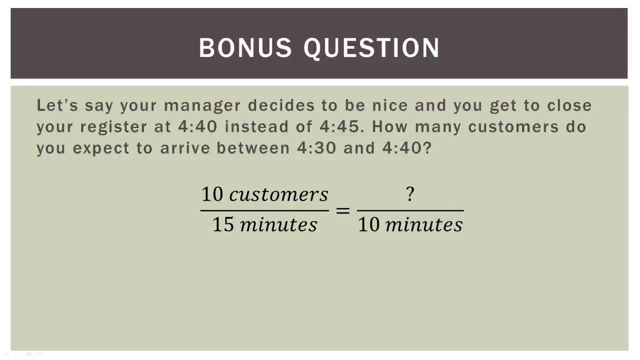 Now that 10 minutes is within that 15,. okay, So it's not outside that 15,, but the 10 minutes within that 15-minute interval. what would we expect? Well, actually, the simple cross-multiply ratio problem, and that is 6.67 customers. 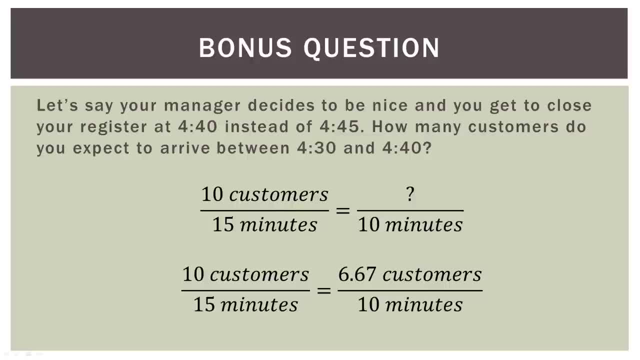 So if we close our register at 4.40, during the 10 minutes from 4.30 to 4.40, we would expect between six and seven customers somewhere in there to come into our line. So if we change the interval, we have to change our. 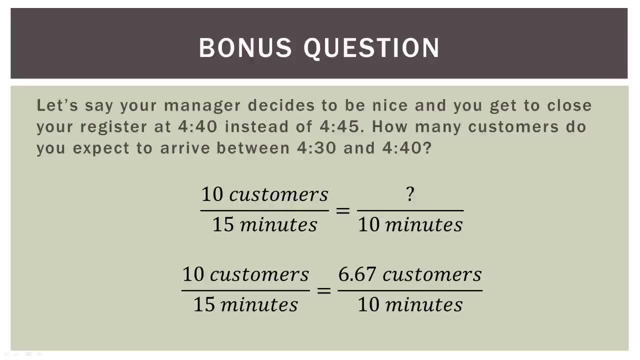 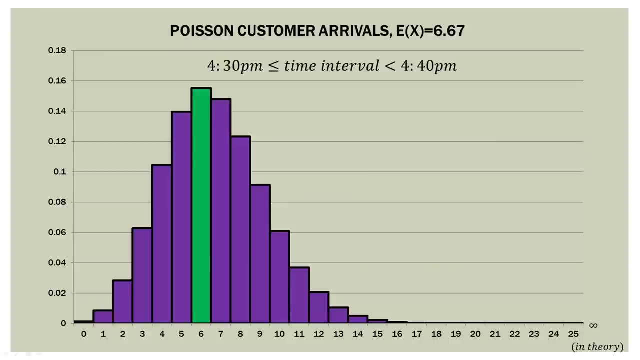 expectation of customers. But again, that 10-minute interval is within our original 15-minute interval and that's very important. So what if we do a graph of this distribution? Well, it looks like this: The time interval is now 4.30 to 4.40,. 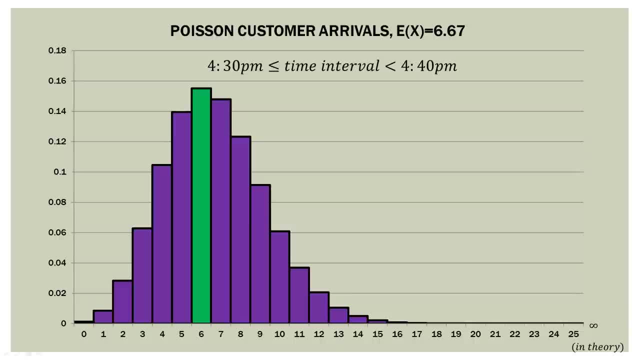 and our expected is 6.67.. So we can use Excel to do this graph and, if you look, the most probable outcome is six customers And the probability of that is over .15 or so .155, something around there. 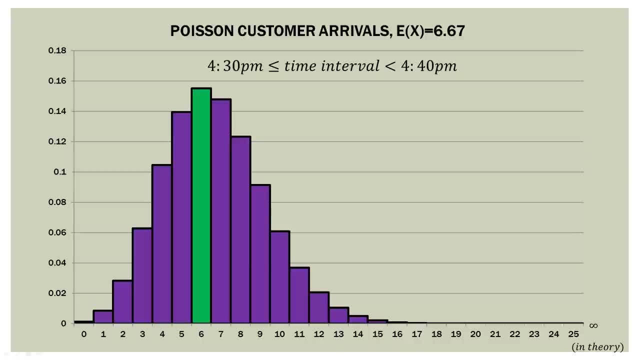 And you can see on either side of that the probability gets lower. So the probability of five is a little bit lower than six, the probability of seven is a little bit lower than six and it falls off from there and looks a very similar shape. 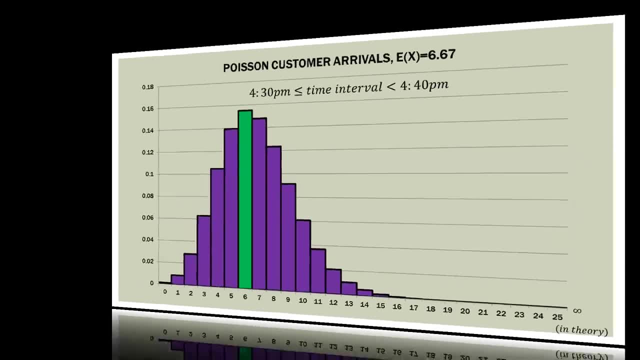 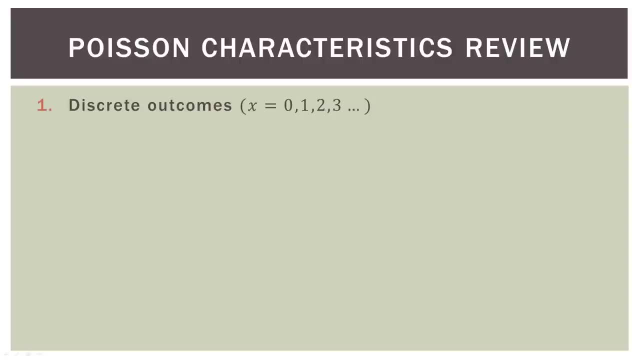 as our previous one. Okay, it's a quick review and we are done. Remember: the Poisson can have discrete outcomes: zero, one, two, three et cetera. The number of occurrences in each interval can range from zero to theoretically infinity. 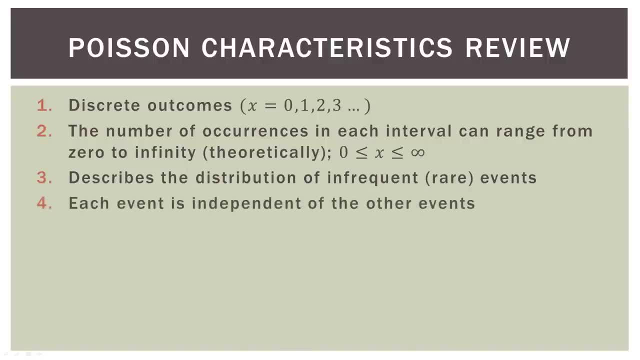 It describes the distribution of infrequent or rare events. Each event is independent of the other event. It describes discrete events over an interval, so an interval of time, distance, et cetera, And that's important. That's sort of what makes a Poisson what it is. 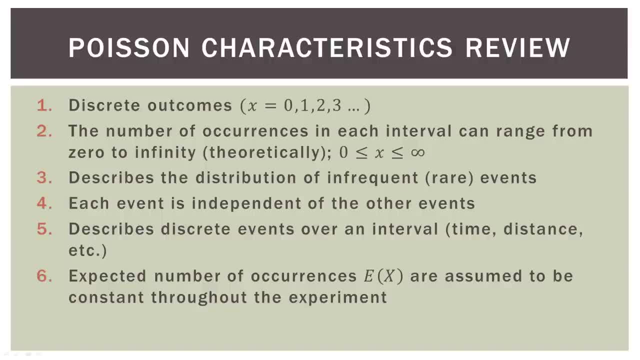 And, finally, the expected number of occurrences are assumed to be constant throughout the experiment, And that's important because of the past question I did in the bonus section, So I changed the interval from 15 minutes to 10 minutes, so 10 minutes within the original 15-minute interval. 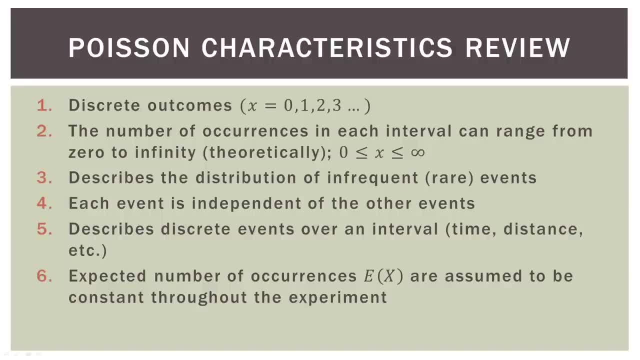 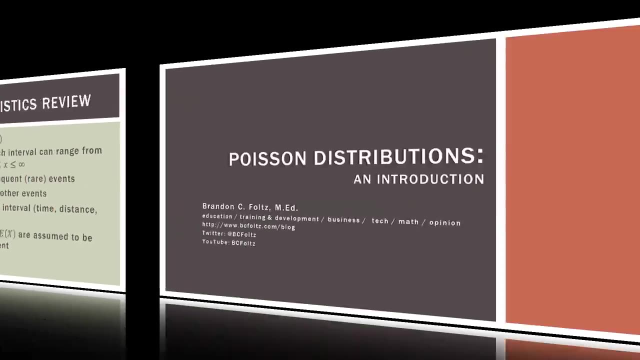 Because I assumed the arrivals into the line were constant. I could do a simple ratio. So again, in real life it doesn't always work that way, but it's a good enough approximation that we can go ahead and make that assumption. Okay, so that is our introduction.